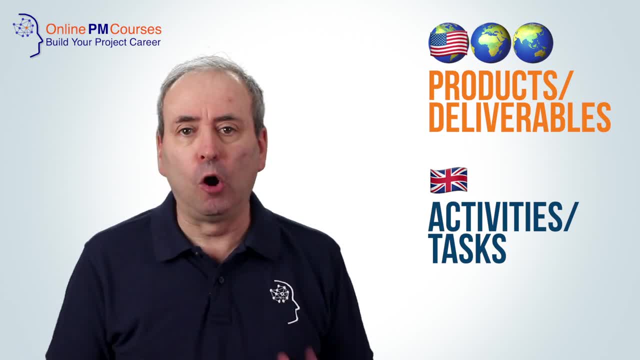 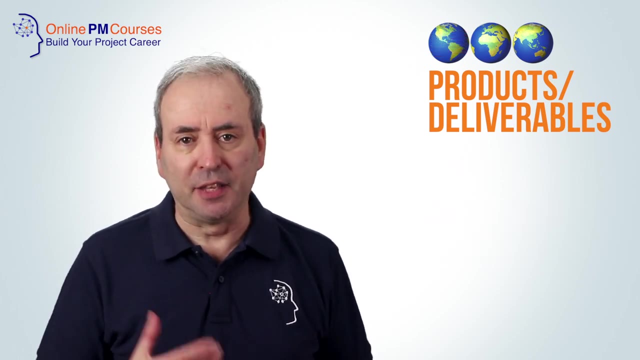 and their adherence, But because it is the more common approach and, some would argue, maybe the more rigorous approach on technical projects, we're going to break down the project into its deliverables to create a work breakdown structure and then use that to identify the tasks that need to be carried out for future planning and scheduling. 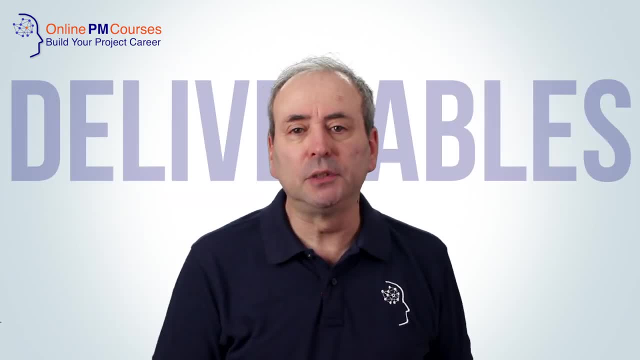 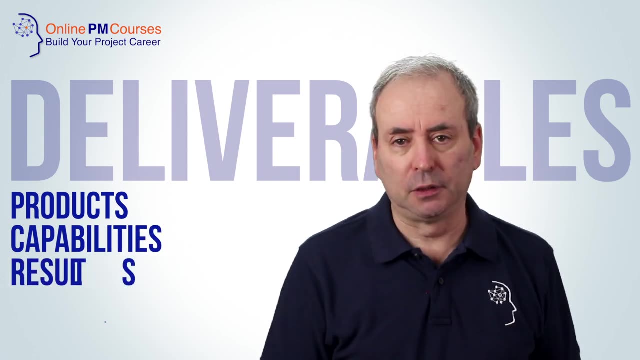 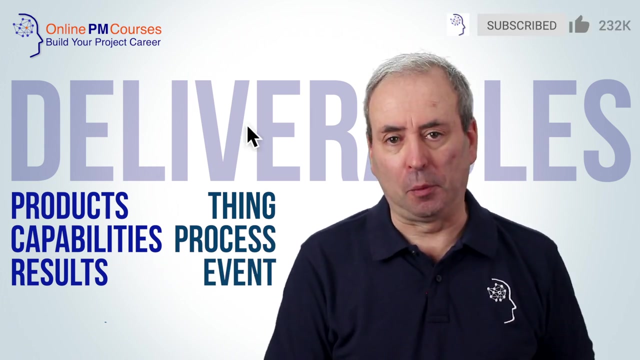 So, because our work breakdown structure is going to break the project into deliverables, let's start by understanding what they are. Deliverables are products or capabilities or results. For example, a thing, a process or an event are deliverables. You could argue that a deliverable is anything tangible that you can experience. 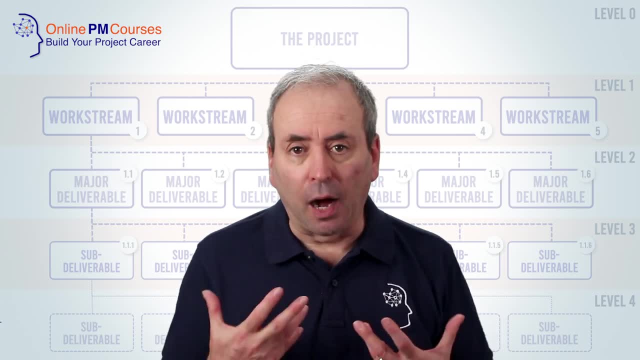 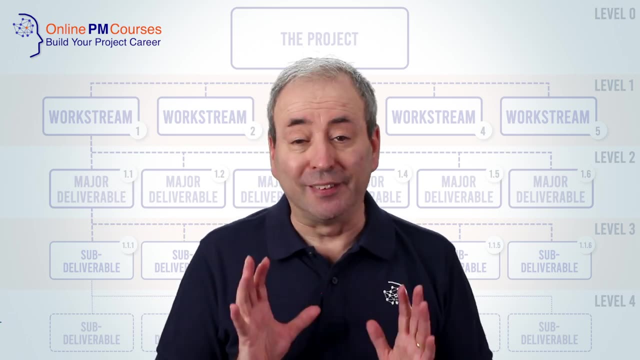 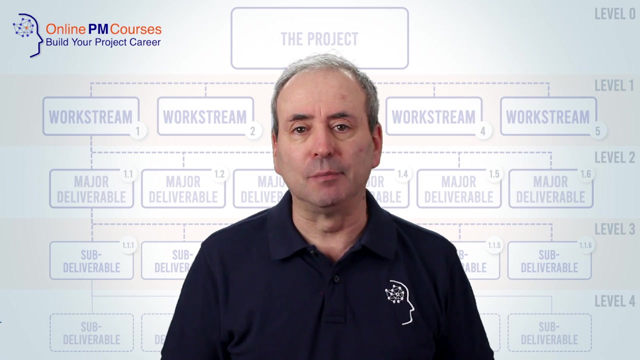 So to create a work breakdown structure, all we need is a hierarchical decomposition of all of the deliverables. and because it's all of the deliverables, it means that if it's not on the work breakdown structure, it won't get done in your project. So it's absolutely crucial that we do it in a systematic way so we don't miss anything. 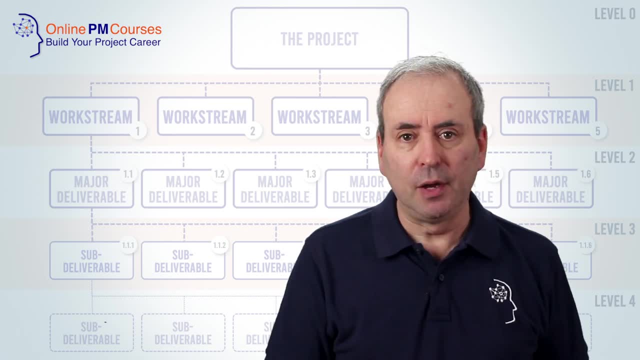 Now you'll find a lot of variance on the process that I'm going to give you, and I don't claim that my approach is any more nor less correct than any others. But what I do want to focus on is being crystal clear about the levels within a work breakdown structure. 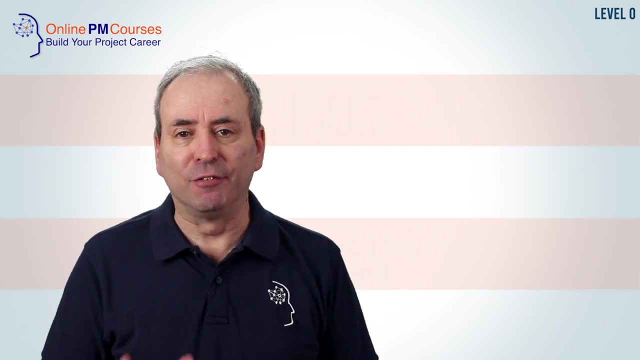 So at the top of our work breakdown structure, we have level zero. This is the product, deliverable or project that we are going to create through the project. It is the totality of the entire deliverable set and therefore the project itself. Level one is what I am going to. 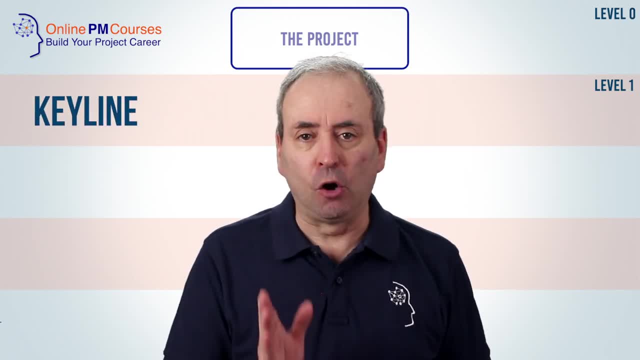 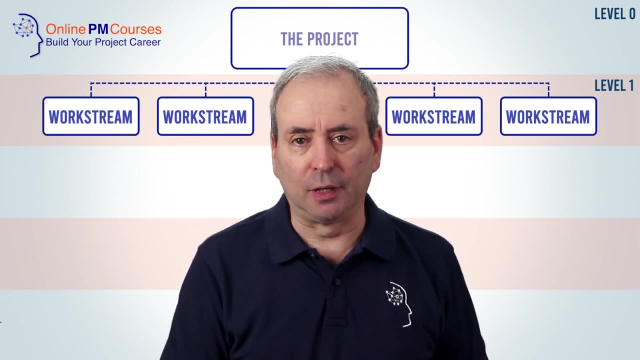 call the key line, and this is not a commonly used term. The key line is our organising principle for the work breakdown structure. It sets up the categories by which we're going to decompose our deliverables. Now, sometimes the key line is nothing more complex than a few deliverables. 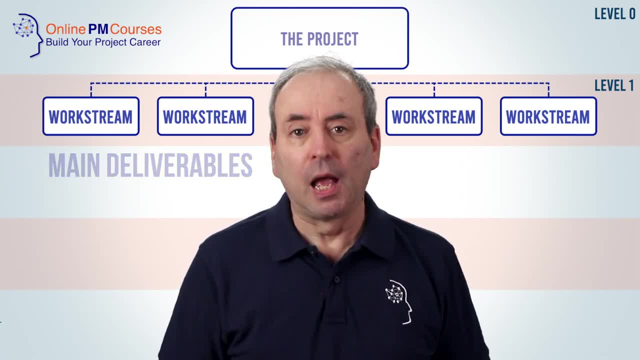 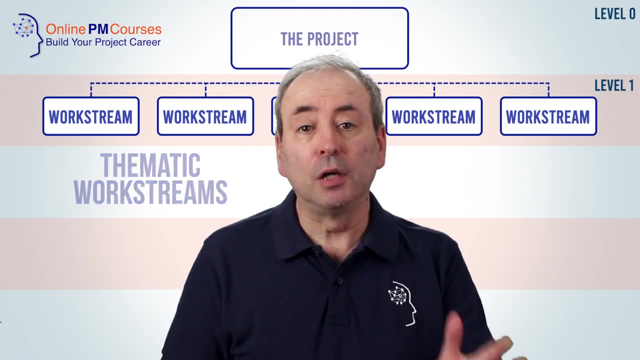 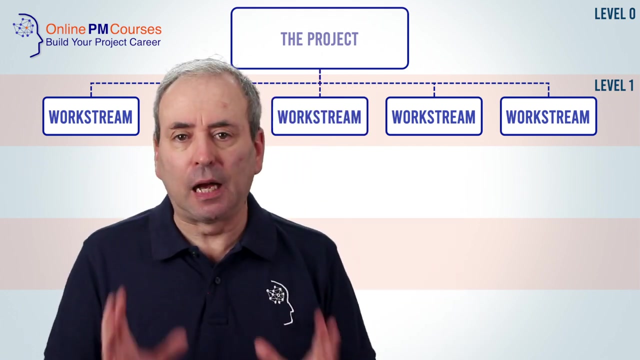 the biggest deliverables of all. In other circumstances, it may be the stages or phases of the project, It may be work streams that are thematic in nature, like technology, people and processes, Or it could even be a geographic set of divisions. However, once you set up the principle against which you're going to decompose the entire project, 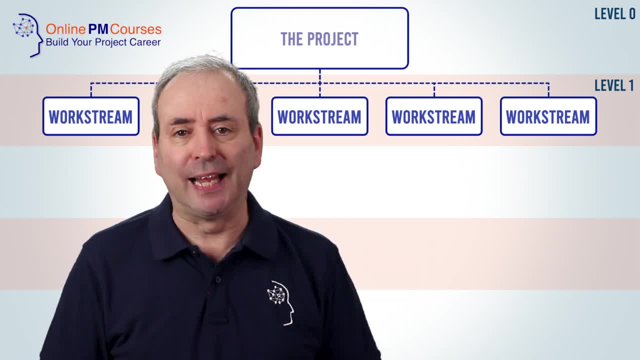 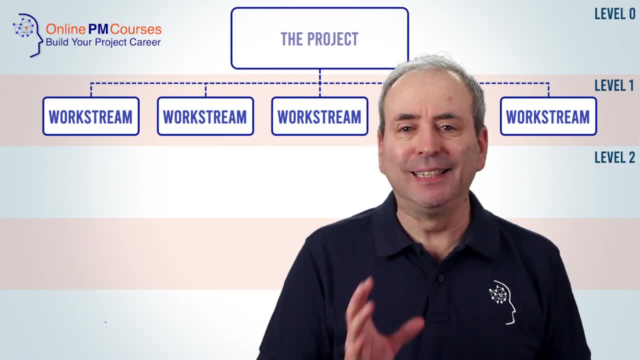 that gives you level one your key line and therefore sets out the titles for the major work streams for your project. Level one is the key line and therefore sets out the titles for the major work streams for your project. At level two, we have the major deliverables that sit within each element of the key line. 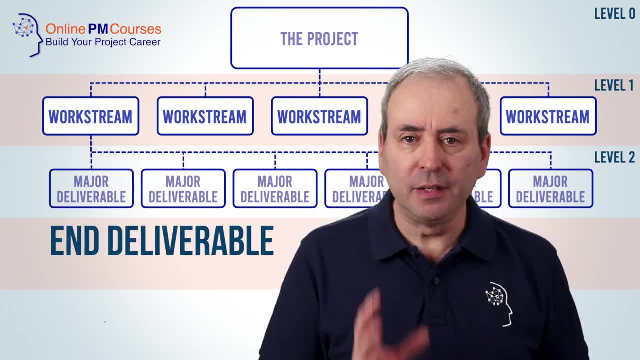 Not all of these deliverables need to be an end deliverable. An end deliverable is something you want. It is there because that is what the project has been created to build. End deliverables are often defined by the goal and the objectives of the project. 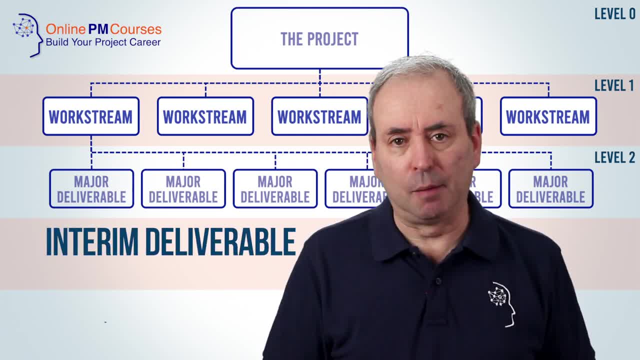 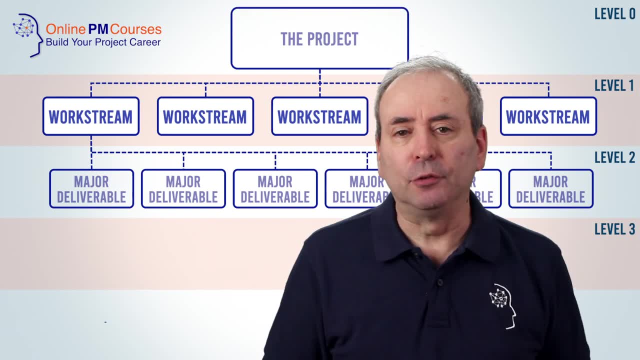 The alternative is interim deliverables, and you may see some at level two, but they are more likely to appear at level three. But while we're at level two, the key here is to use expertise- the experts on your project team- to identify the major end deliverables and the major interim deliverables. 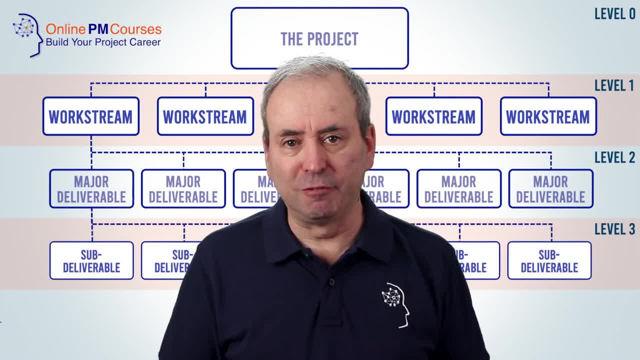 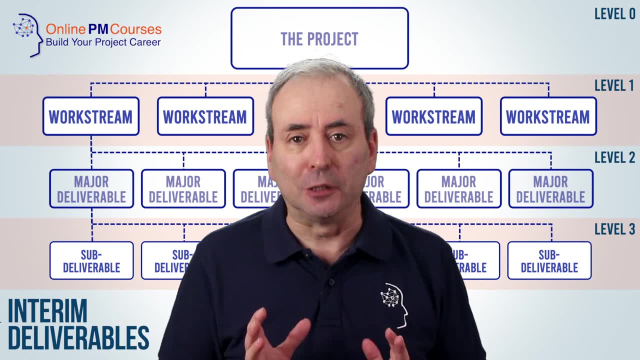 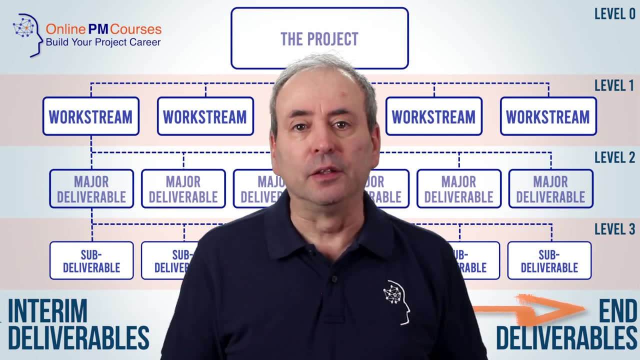 So at level three, we will see components of the major deliverables and we will see a large number of interim deliverables. Interim deliverables are things we need to create in the project in order to help us get to the end deliverables. Typically they include things like prototypes and tests. They include project management artefacts. 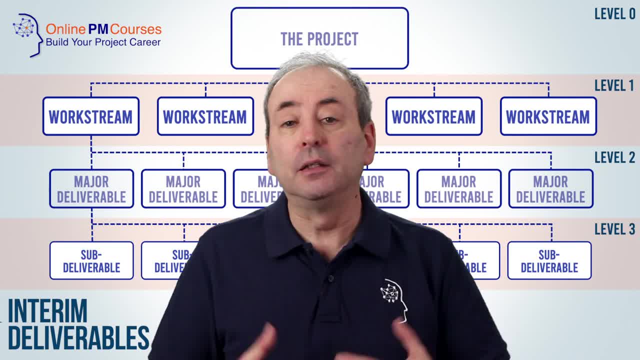 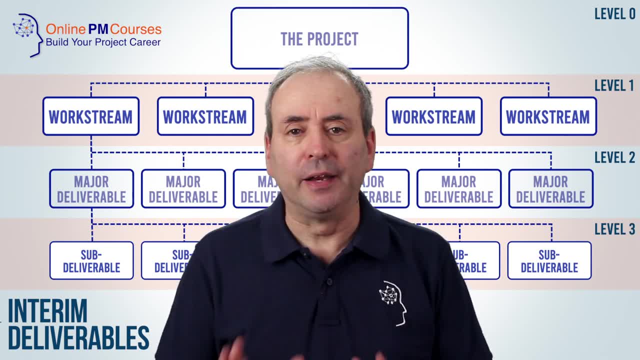 like plans and stakeholder lists. They include things like test scripts and maybe even components that we don't need but that will find their way into the end deliverables. So, to create level three, we need to brainstorm the sub-deliverables that we need to create in order to get to the end deliverables. 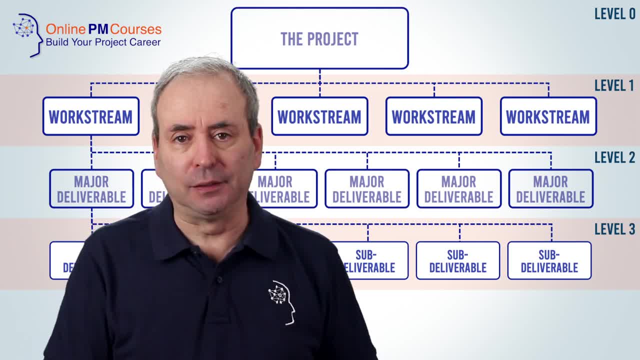 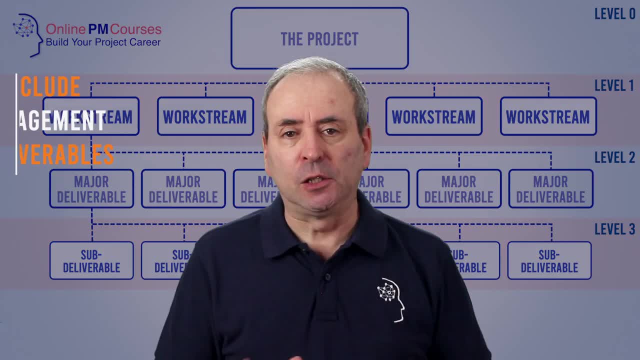 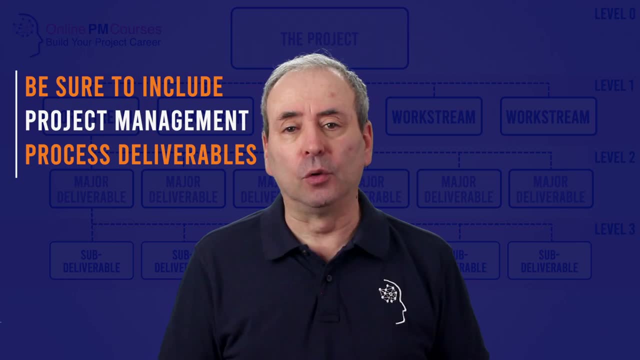 And the interim deliverables for each of the items at level two. Remember, because if it's not on the work breakdown structure, it won't get done- be sure to include project management process deliverables, the artefacts of project management. And one way to do that, of course, and my preference, is to set up a project management. 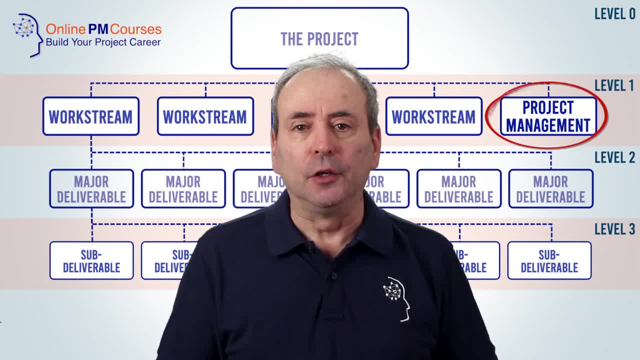 heading at the key line level. That way, you can decompose your approach to project management into a number of major and then sub-deliverables at levels two and three. Remember, everything in this work stream will, of course, be an interim deliverable by definition. 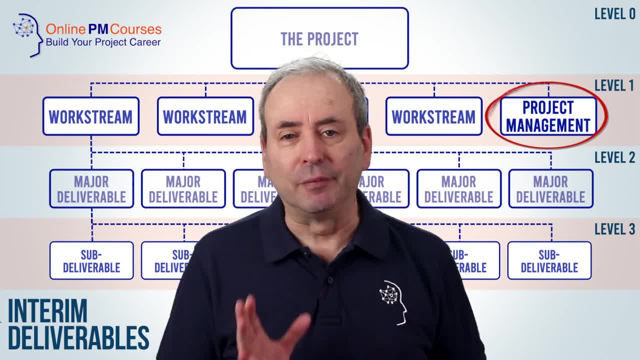 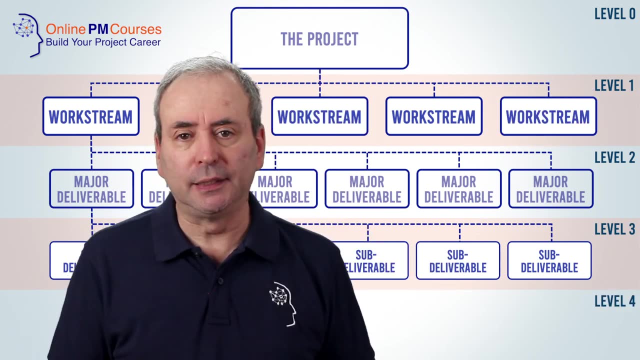 because it's not something we want as an end product. it is something we need to create along the way. If you do create this project level work stream at the key line, typical names would be project management or project integration. Level four and maybe levels below this further decompose the sub-deliverables and the interim. 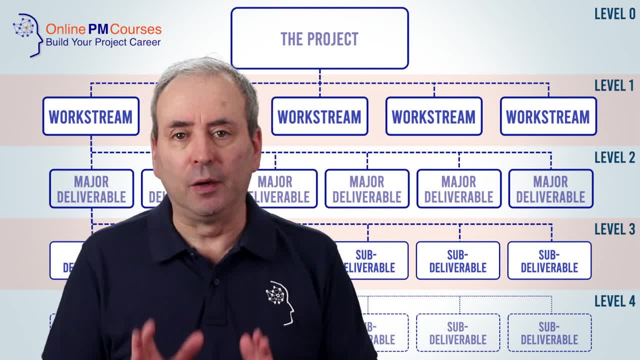 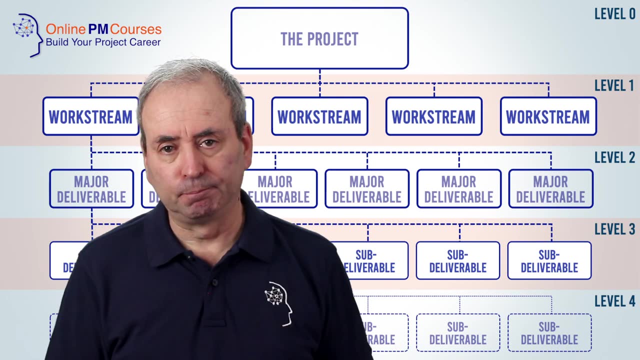 deliverables into smaller and smaller deliverables, to the point where each deliverable is a unique and fully constrained thing in itself. Make sure that these are structured into logical hierarchies and, as far as possible, sequenced in a logical order, And of course it may not look tidy, but it is okay. 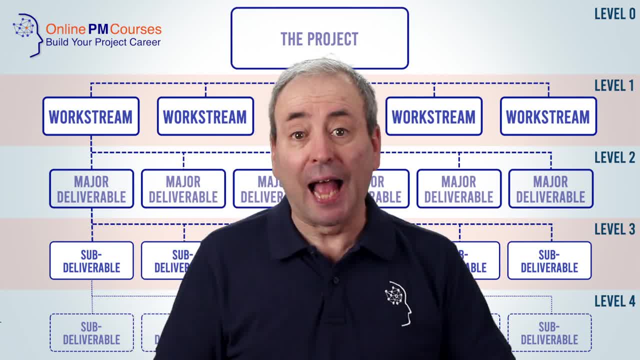 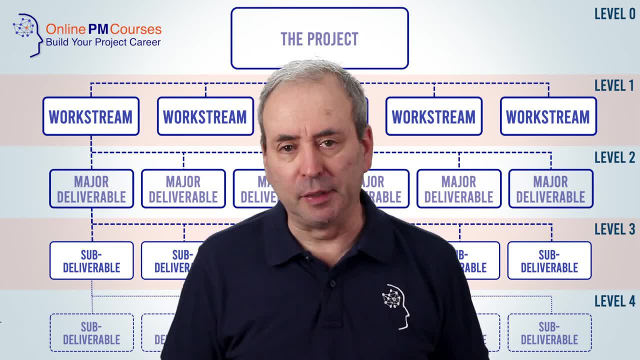 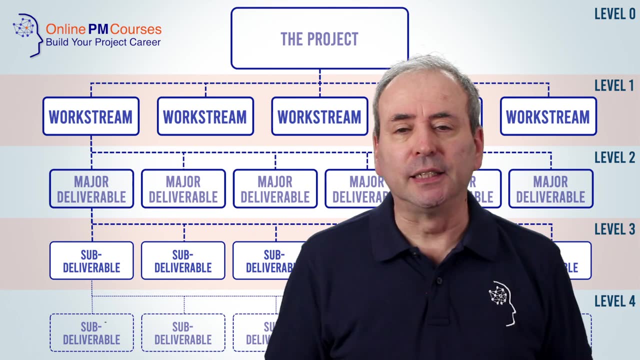 to go to different depths, different numbers of levels at different parts of the work breakdown structure, because your work breakdown structure should be determined by the work that needs to be done, not by some platonic ideal of a perfect, neat work breakdown structure. The next thing to do is: 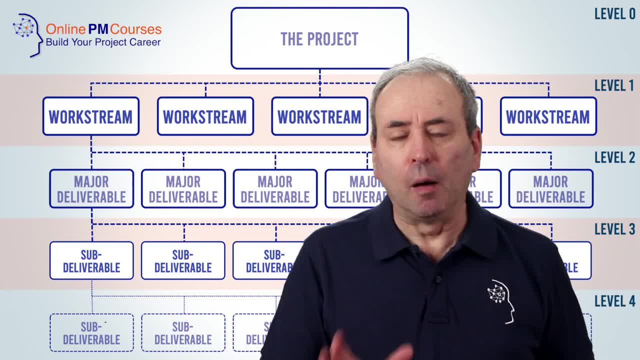 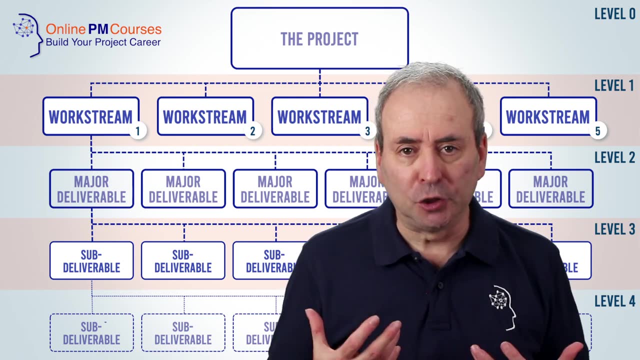 to document your work breakdown structure. We start by creating a work breakdown structure index. We number one, two, three, four, five and so on across the key line. Then, starting with the first element, we look at the sub-deliverables on line two and we number them. 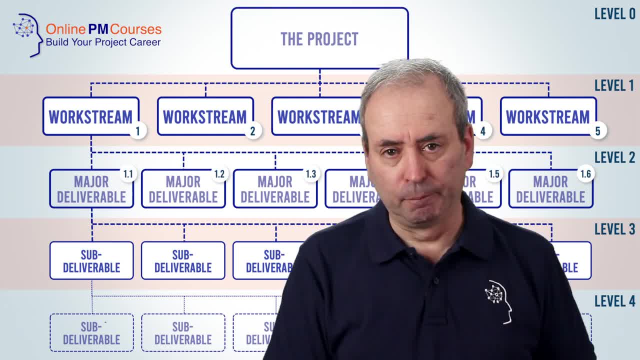 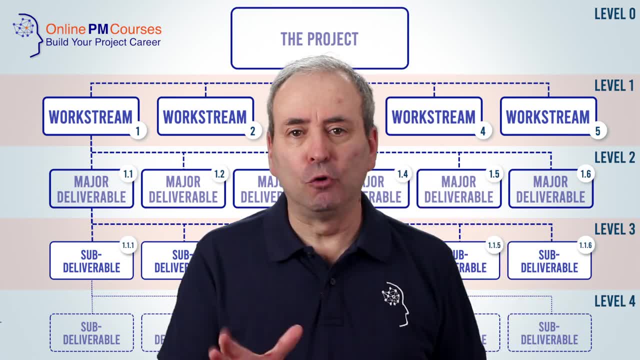 1.1,, 1.2,, 1.3 and so on. Every item on your work breakdown structure will have an index number in that format, and that format should look very familiar to you because it is very easy to create a work breakdown structure using a simple word processing package like Word or Pages. 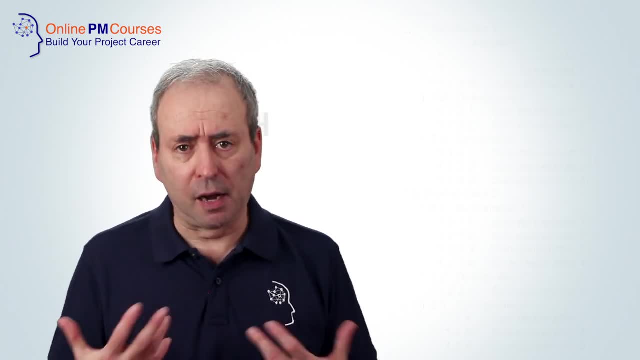 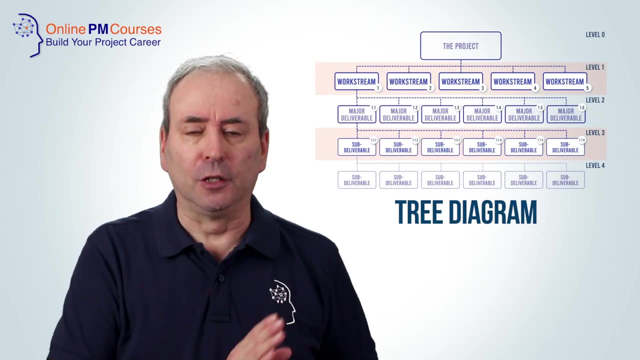 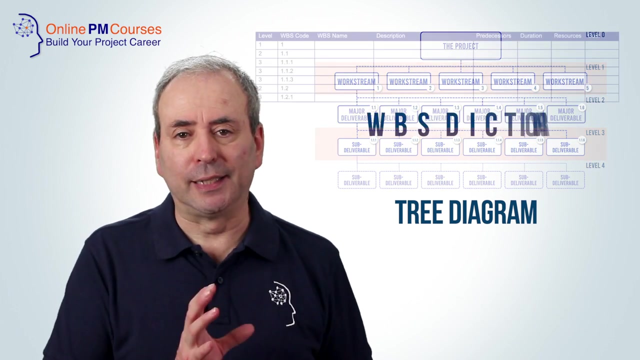 You have a number of ways that you can present this. You can present it as a hierarchical list or as a tree diagram, which is commonly presented as particularly in a training context, but for a large project is rarely practical. Or you can create a work breakdown, structure dictionary. 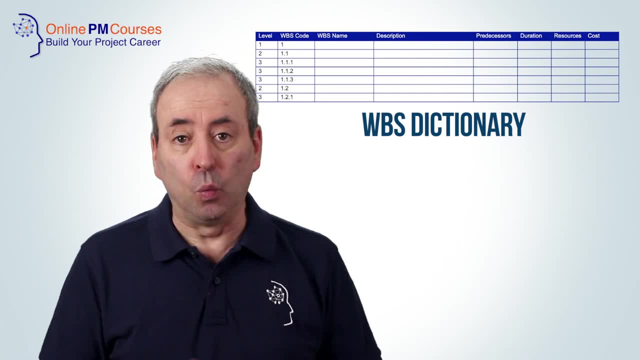 a WBS dictionary which lists every product with its reference number, but now you can add additional information. You can add descriptions. You can add descriptions, Standards, specifications. you get feedback on it and refine it, bring it right: standards, specifications, resources, costs, durations and anything else that 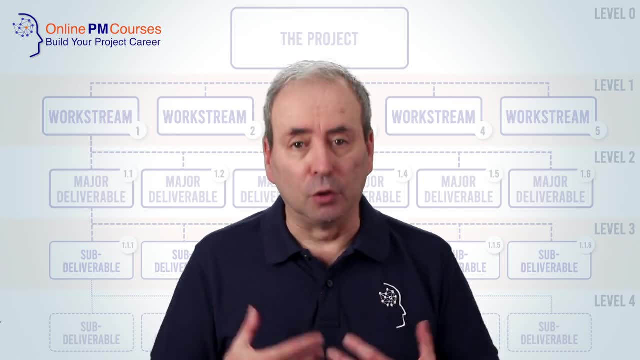 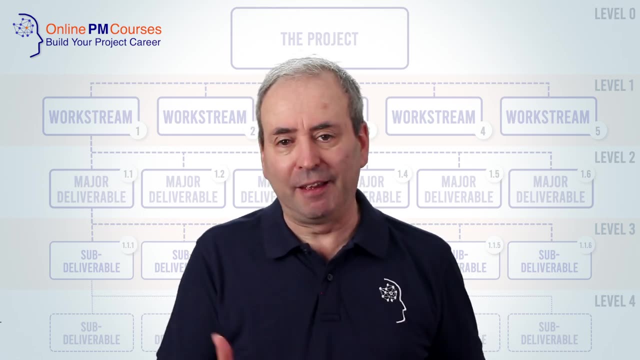 is relevant to you to create your work breakdown structure dictionary. The final step is to present your work breakdown structure to your project sponsor, to your client, your boss, to your steering group and, indeed, to your stakeholders. Get their feedback on it and refine it before producing your final version. 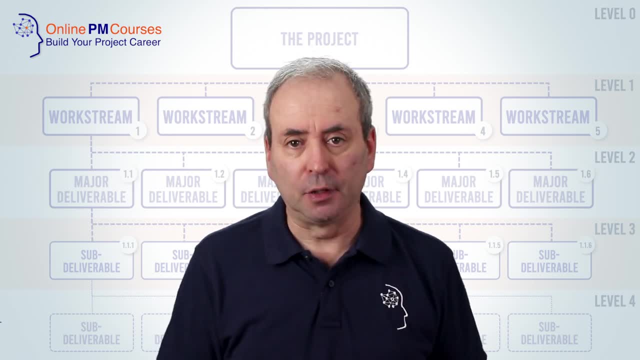 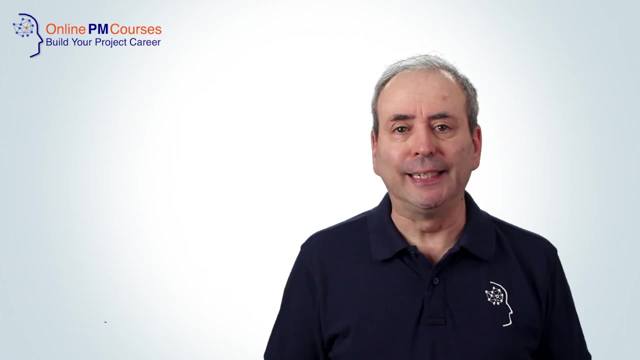 breakdown structure is now a full and formal statement of the complete scope of your project. Before we turn our deliverable-based work breakdown structure into an activity tool that we can use for planning and scheduling, let's look at some good practices in creating your work breakdown structure. First, make sure the labels of each item in 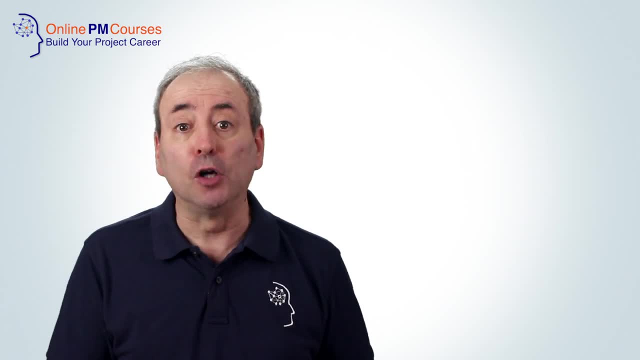 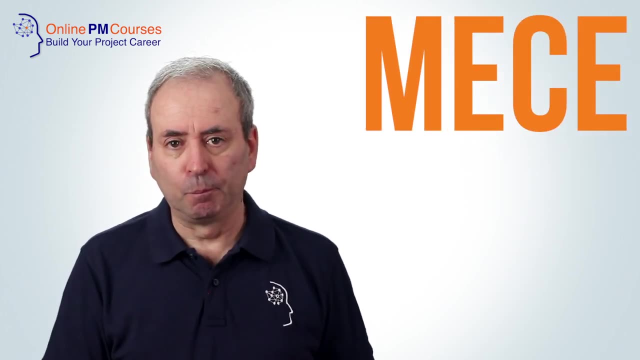 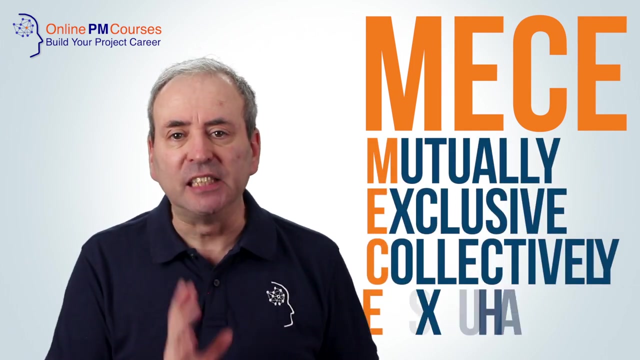 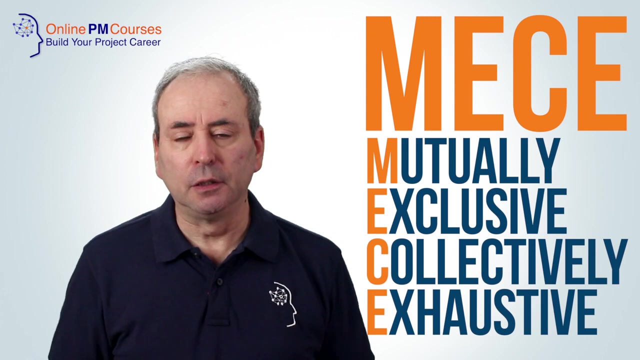 your work breakdown structure provide a clear and unambiguous description of what that deliverable is. Secondly, apply the Mies Principle: Is your work breakdown structure mutually exclusive and collectively exhaustive? What do we mean by mutually exclusive and collectively exhaustive? By mutually exclusive, we mean there are no overlaps and that the same deliverable doesn't. 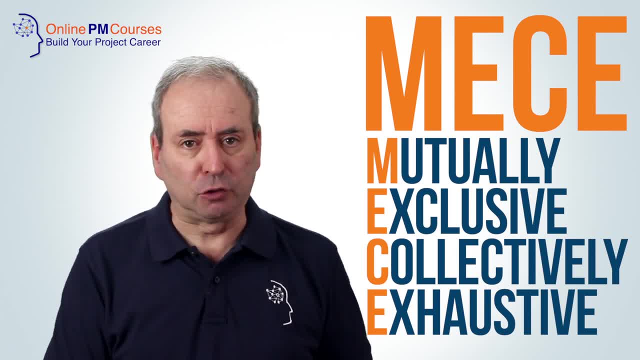 appear twice or more times in different parts of the work breakdown structure, and by collectively exhaustive we mean there are no overlaps. By mutually exclusive we mean there are no overlaps and that the same work breakdown structure, a part of it is. So this is a kind 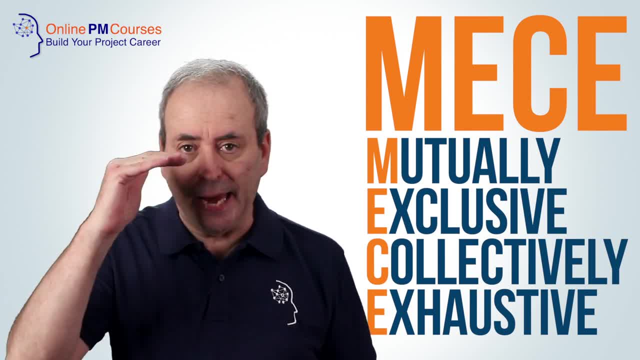 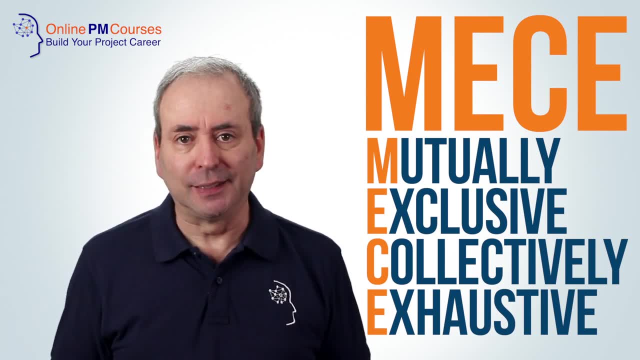 we mean that any deliverable at a level can be completely specified by all the sub deliverables below it. That is to say, that the entire work breakdown structure does indeed represent the complete project and everything you need, both your end deliverables, the components of the end. 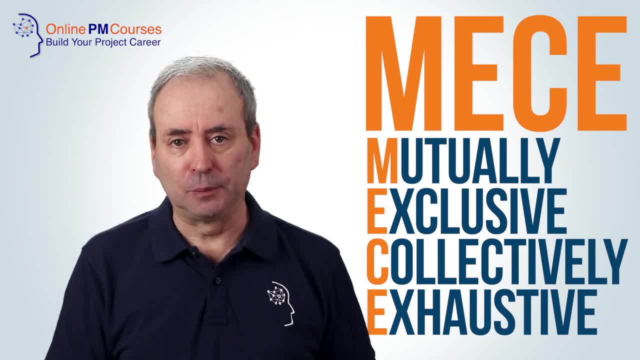 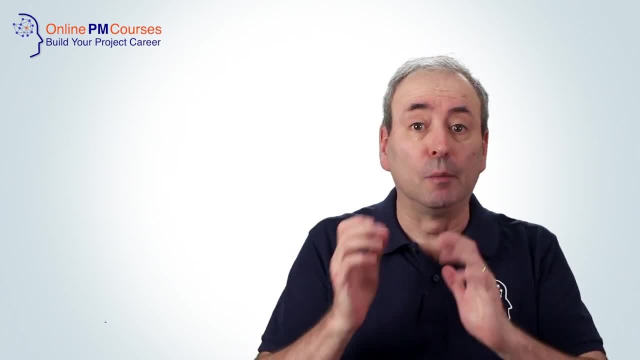 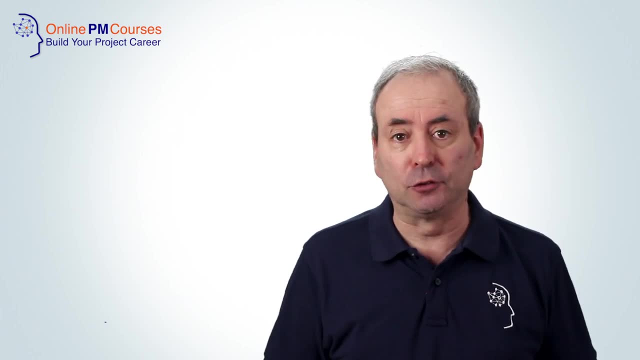 deliverables and your interim deliverables. Now, it's worth noting that on many modern projects, where they are moving from a purely predictive to a more hybrid style of project management, it isn't always going to be appropriate to try to complete the work breakdown structure at the start of the project. The project may evolve and you may need to add elements, or indeed, 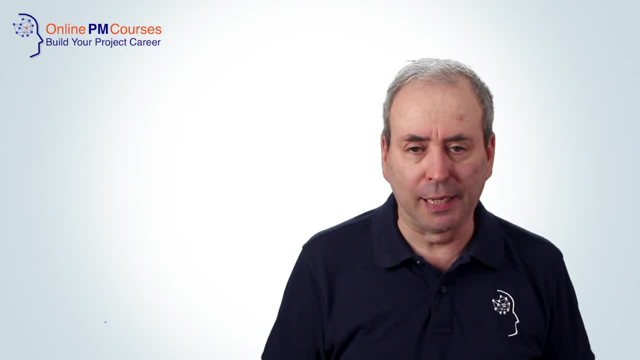 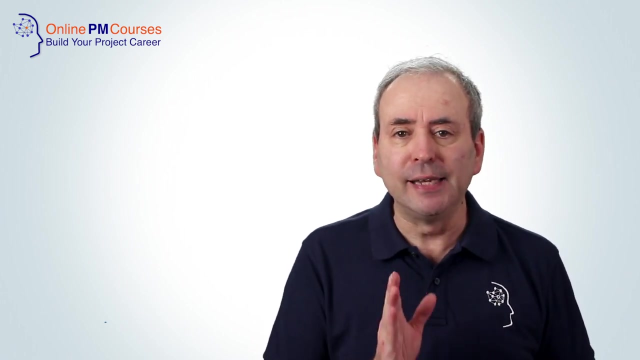 delete elements from your work breakdown structure. as you go through the project, discover new requirements, learn more about the project you're doing. So whilst I grew up in a predictive environment where we would create a full work breakdown structure before moving out of the planning phase into delivery, that isn't necessarily going to be your approach. 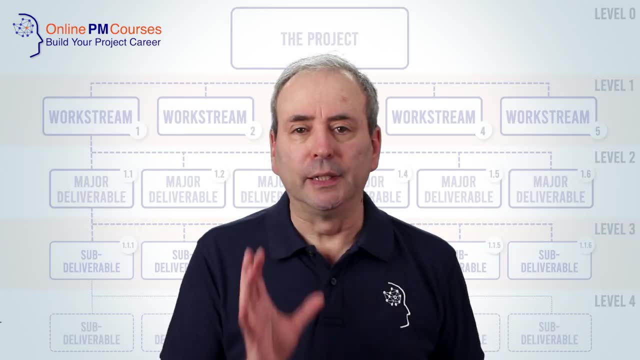 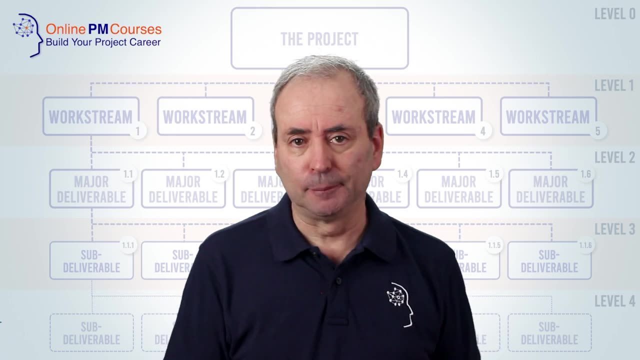 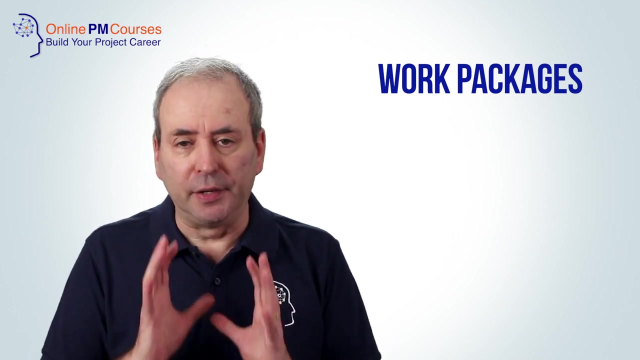 in every project. Now you've got your deliverable based work breakdown structure, how do you understand the tasks, the activities it takes to create your project? The first step is to create work packages to identify deliverables or groups of deliverables that need to be created together and set up work packages that collectively develop those. 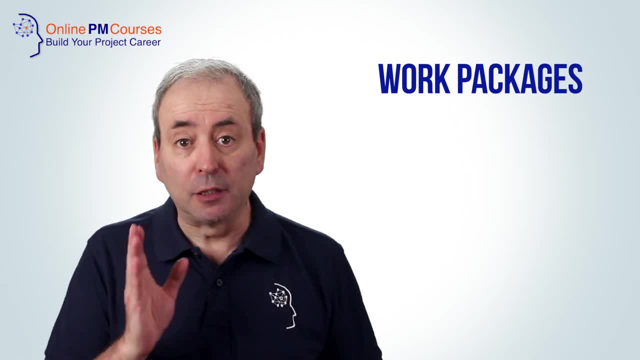 deliverables. Typically, you will have one work package create one deliverable, but that won't always be the case. and also typically you will allocate the task of creating this work package decomposition to your work stream leaders who understand the tasks and the deliverables within their 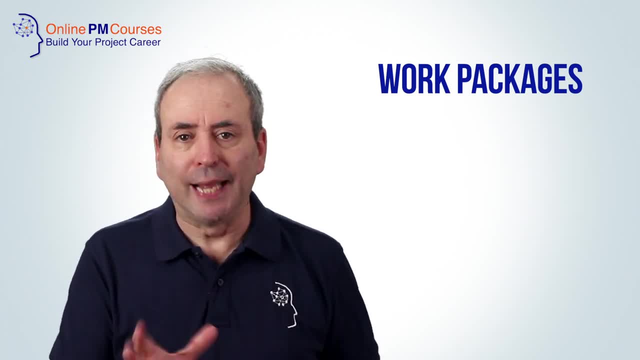 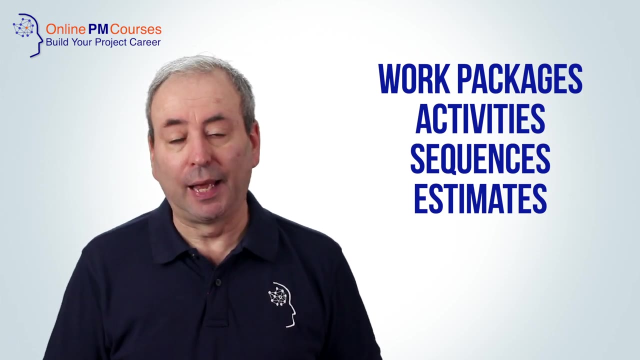 work stream better than you do. Once they've created the work packages, they will decompose those into the individual activities that need to be done. These can be then arranged into logical sequences and you can estimate time and resources against them and indeed budget for them. And that's the third step. Planning is about taking the sequence of activities. 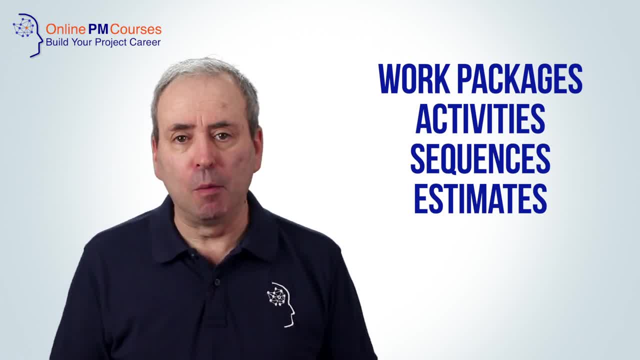 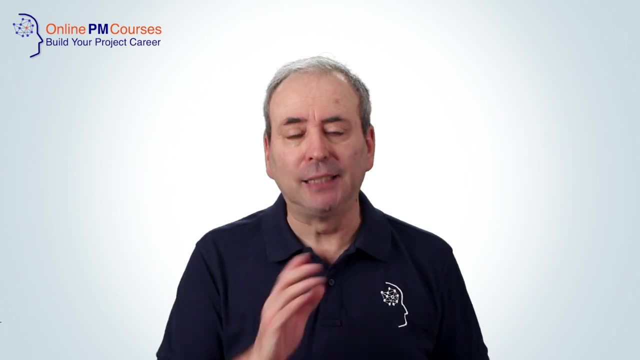 that you identified, taking the estimates of how much work it takes to deliver them and the duration of those activities and putting them into a schedule and building a budget. So, from a work breakdown structure, you can determine the dependencies, estimate durations, allocate resources into those tasks and, therefore, 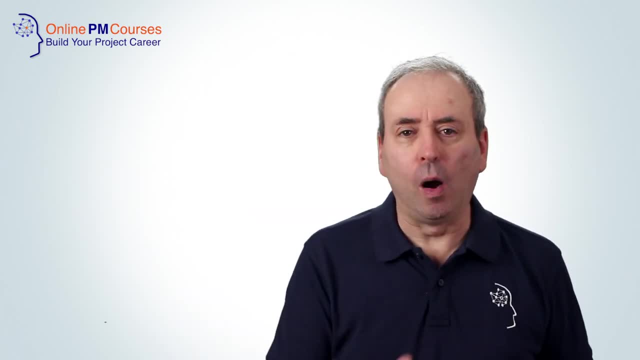 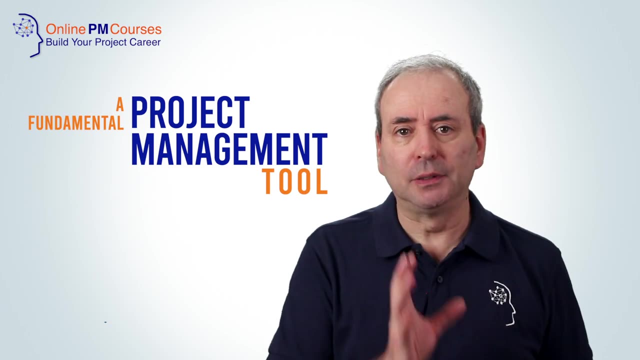 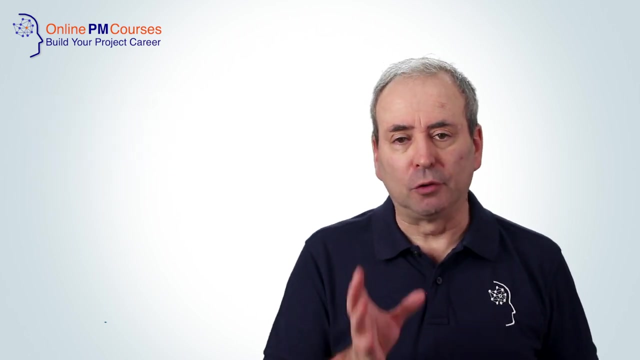 estimate costs. So now I hope you can see why I describe work breakdown structure as a fundamental project management tool. it's the tool that opens up the way and connects with so many other project management artefacts. The work breakdown structure is a scoping and scope management tool. It's a